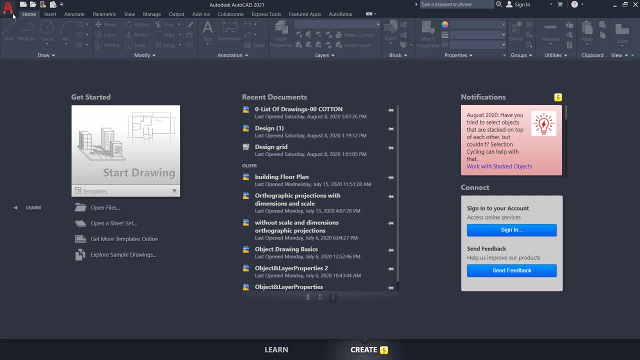 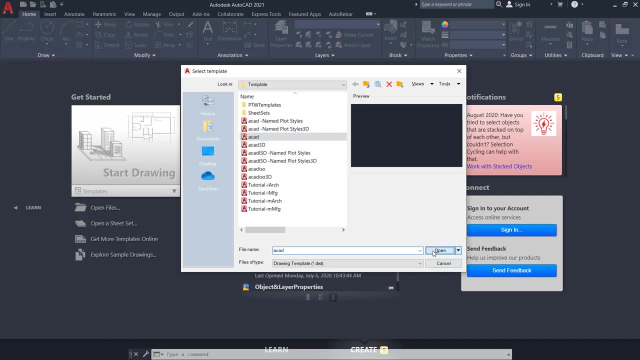 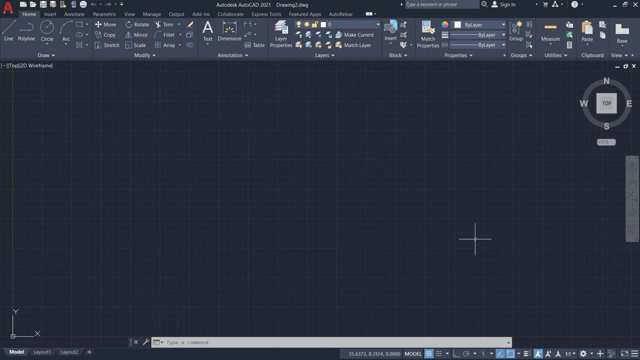 For AutoCAD 3D: start from a new file- New- Okay. Here I will select AutoCAD. Okay. When we open the new file in AutoCAD it automatically comes with the workspace drafting and annotation. That is the basic drawing phenomena in AutoCAD. 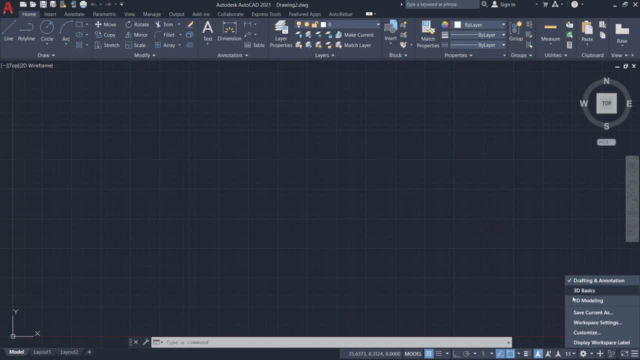 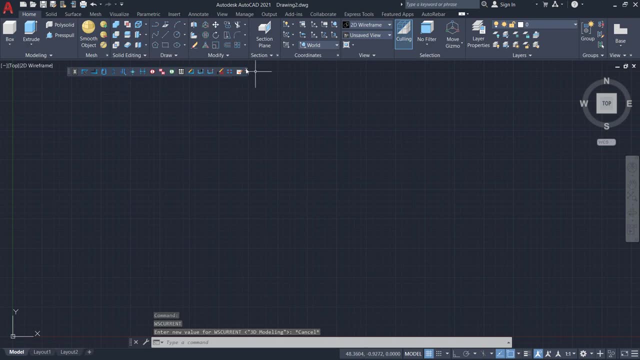 To draw the 3D modeling we have to select 3D modeling, Then the tabs of 3D will appear Here: Box, cylinder, cone- We directly draw the 3D objects. Okay, In this drawing I will show from the basics as a beginner level. Okay, First of all, here, unsaved view, You can set any view, Like southeast view, top view. 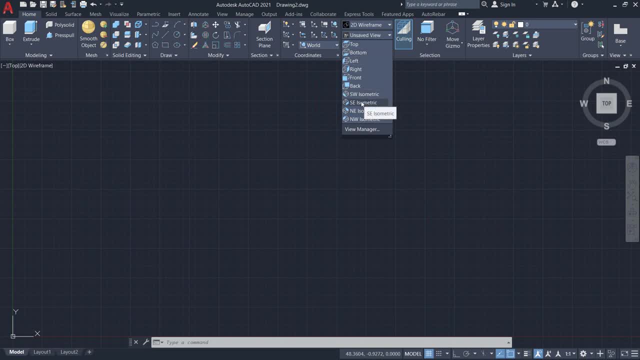 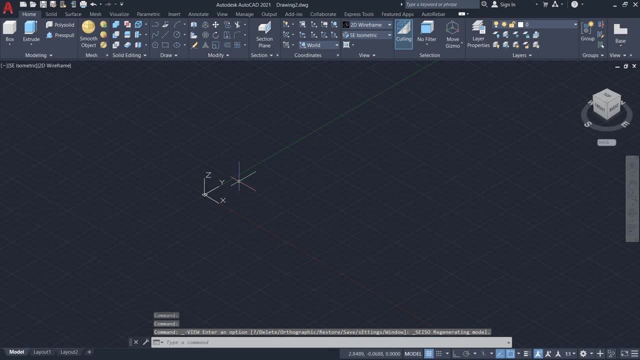 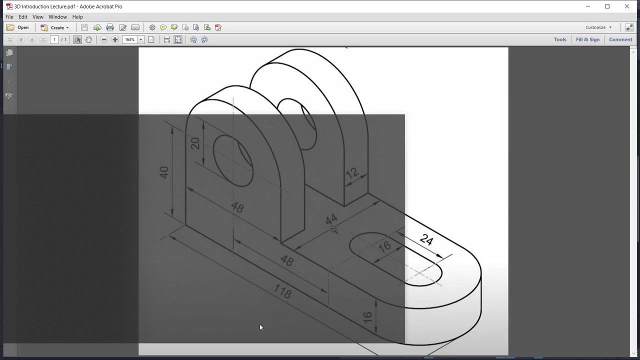 bottom view. So in this drawing I will select southeast. You can select as per your requirement. Okay, That is a 3D view. Now I will select a simple rectangle command, or you can use any line command for drawing the rectangle. Why I am drawing the rectangle In this drawing? I will show you how to draw this 3D object whose length is 118 and 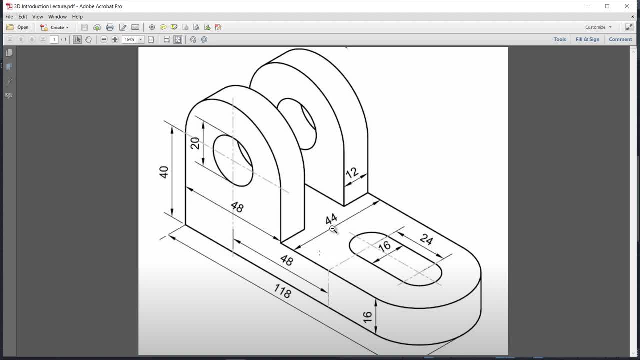 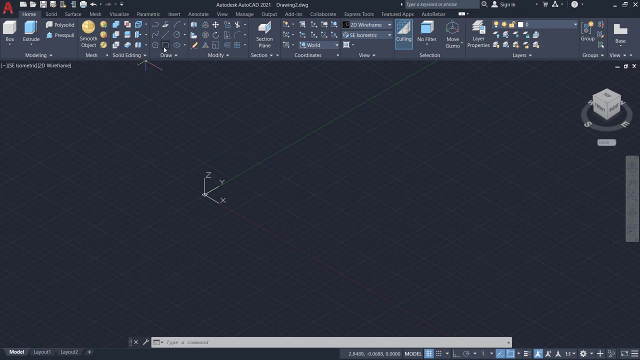 whose height is 40 and whose width is 44. And this little projection height, that is, 16.. Okay, First of all I will draw the bottom portion, Then I will draw the top portions. So, for drawing the bottom portion, 118,, 44 and 16.. Okay, I will select rectangle. Okay, Select any point. 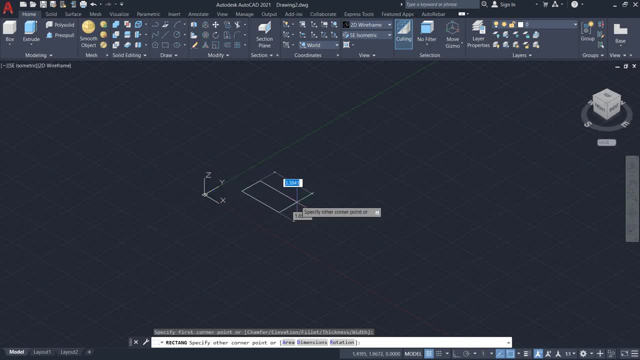 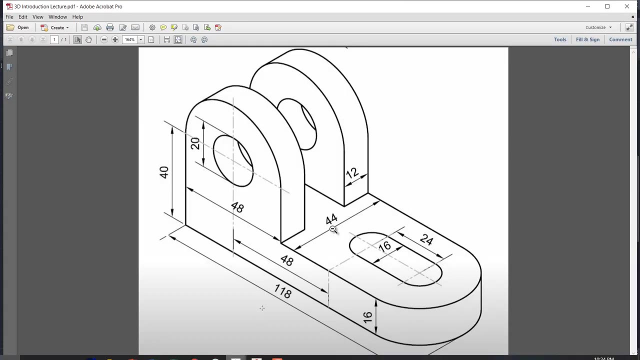 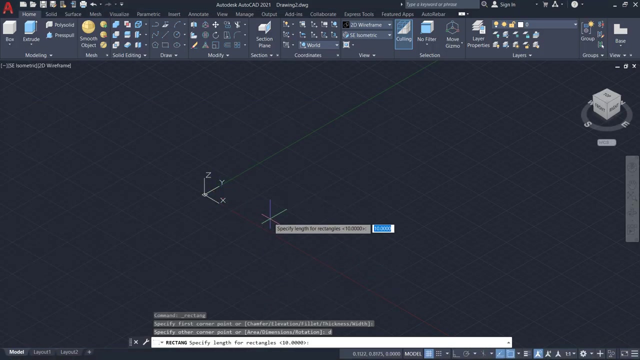 Okay, I have selected any point. Now I will press dimension. Okay, In the dimension I will enter the length and width. I will enter the length, that is 114.. Sorry, 118 and width is 44.. 118, that is the length and width is 44.. I will press enter. 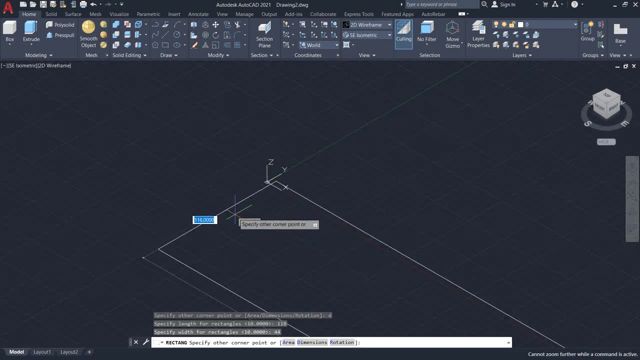 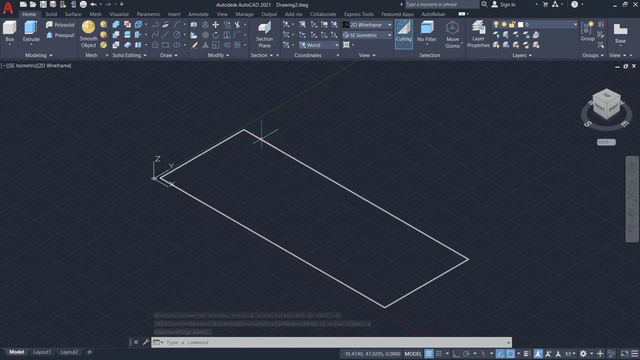 okay, on which side I want to draw the drawing? okay, I have selected this side. now press Z for zoom. for press a for zoom. all okay, now that's the rectangle. now I will project upward to make the height of 16. you have to just use the. 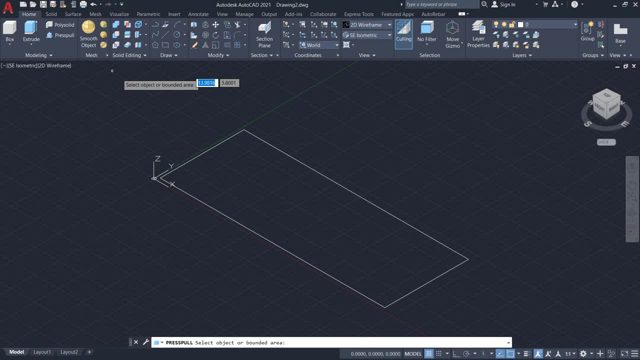 command, press pull. okay, here, press pull, select the object. okay, then press the height which you want. so the height in the drawing that is 16. okay, so I will enter 16. okay, so to view in the 3d, 3d form. so here the by default 2d wide. 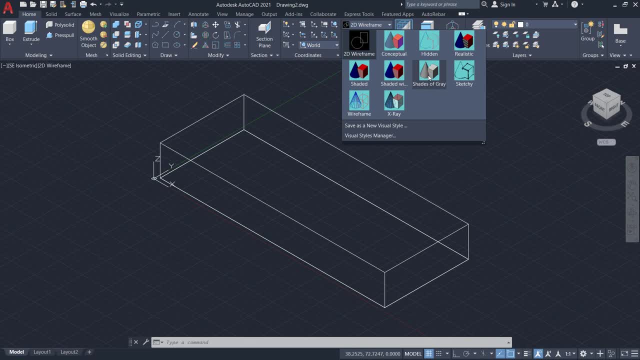 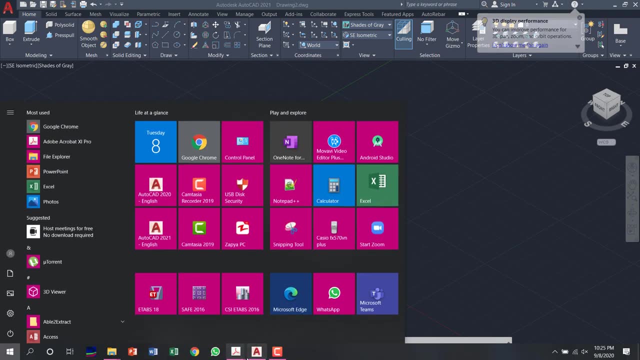 frame is open, so I will select shades of gray. okay, so I will select shades of gray. okay, so I will select shades of gray. now you can see 3d object is looking. okay. now you can see 3d object is looking. okay. now you can see. 3d object is looking okay. now for the curve for this portion. 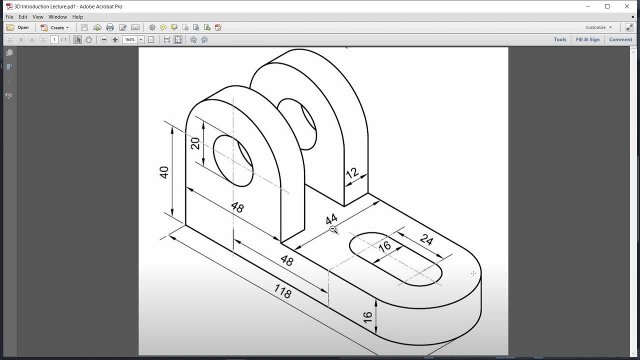 now for the curve for this portion. now for the curve for this portion. okay, the width is 44, so the dia of this. okay, the width is 44, so the dia of this. okay, the width is 44, so the dia of this circle which is curving outside, that is. 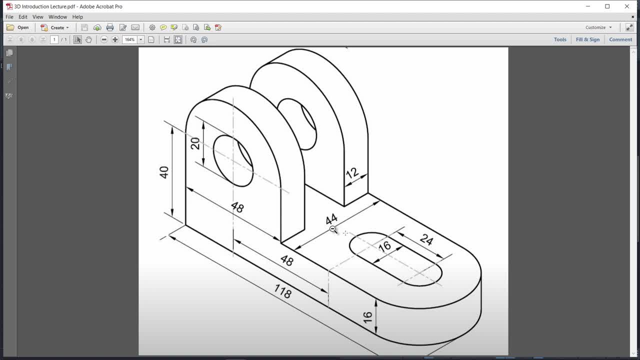 circle which is curving outside. that is circle which is curving outside. that is 44, and the radius that will be 22- okay, 44. and the radius that will be 22- okay, 44, and the radius that will be 22- okay. so, first of all, I will make a line. 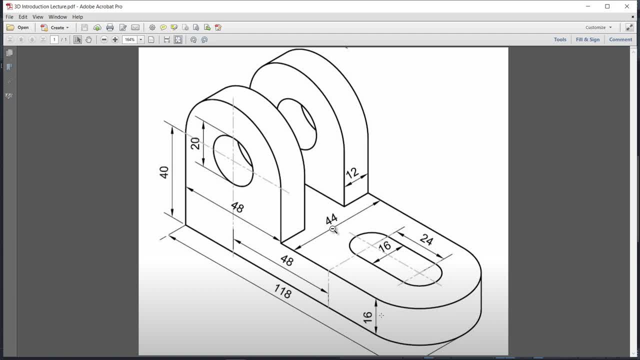 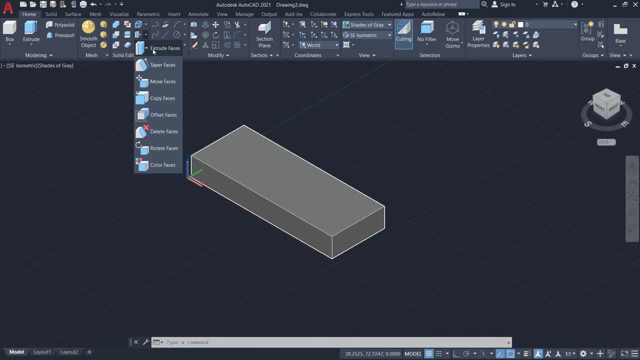 so, first of all, I will make a line. so, first of all, I will make a line, reference line at this point, to draw the reference line at this point. to draw the reference line at this point, to draw the circle, okay, circle, okay. here I will- here is the options- extrude faces. 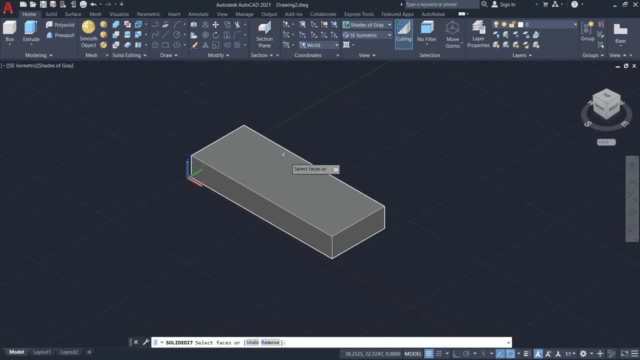 here I will. here is the options extrude faces. here I will. here is the options extrude faces: Tapper faces. I want to copy face- Tapper faces. I want to copy face- Tapper faces. I want to copy face- okay. I want to copy this face. okay, and. 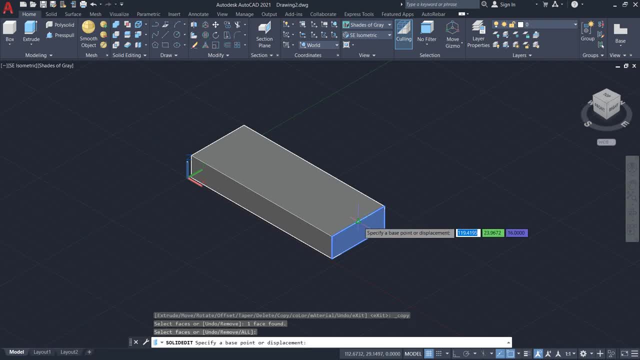 okay, I want to copy this face. okay, and okay, I want to copy this face. okay, and select: enter, then select from where you select. enter, then select from where you select. enter, then select from where you want to copy and locate. okay, so I snap. want to copy and locate? okay, so I snap. 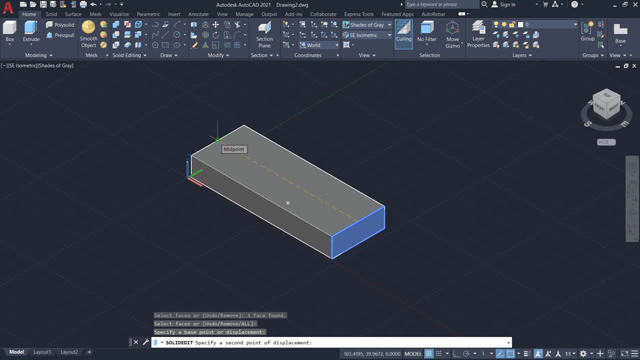 want to copy and locate, okay, so I snap by because it comes in the linear by, because it comes in the linear by, because it comes in the linear position. so now I will enter 22 okay position. so now I will enter 22 okay position. so now I will enter 22 okay, exit. 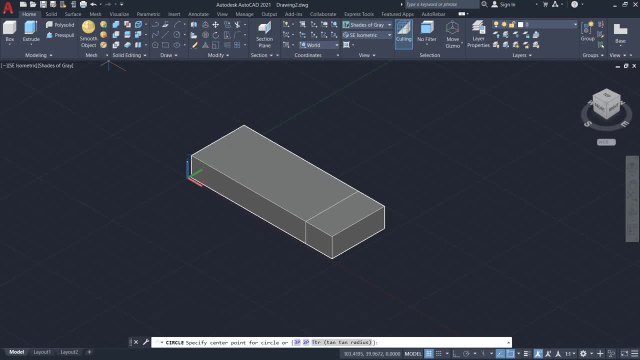 exit, exit. now I will draw the circle. that is circle. now I will draw the circle that is circle. now I will draw the circle that is circle. whose die is 44: okay, here. I have. whose die is 44: okay here I have. whose die is 44: okay here. I have selected Center point. I will select at: 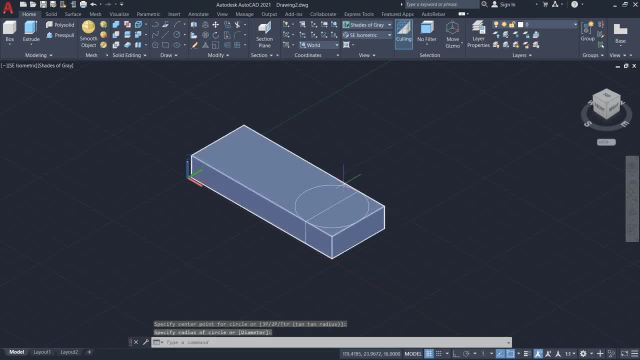 selected Center point. I will select at selected Center point. I will select at the edge. so here is it a circle 44, so the edge. so here is it a circle 44, so the edge. so here is it a circle 44, so now at the edges. I do not need this part. 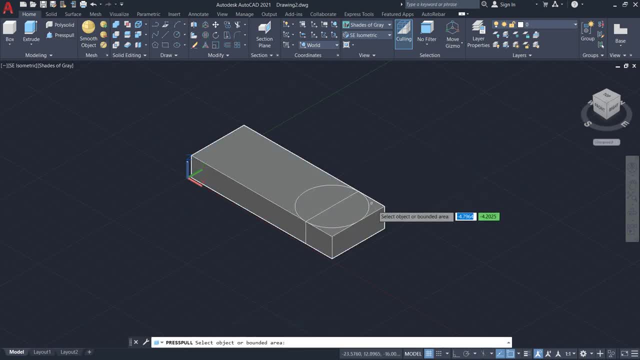 now at the edges. I do not need this part. now at the edges, I do not need this part. so I will just select, press and pull. so I will just select, press and pull. so I will just select, press and pull, select this outside part and go down. okay. 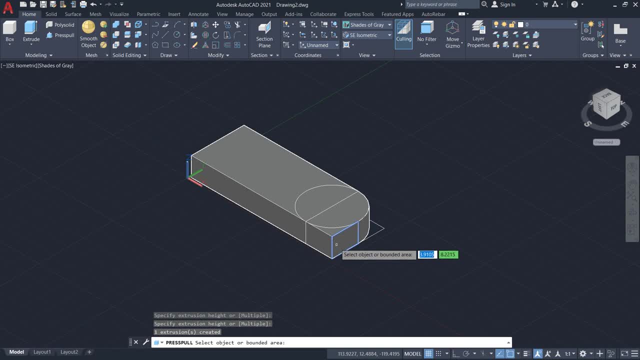 select this outside part and go down. okay, select this outside part and go down. okay, you can see now the outside part is. you can see now the outside part is. you can see now the outside part is deleted, deleted. so again I will select. deleted, deleted, so again I will select. 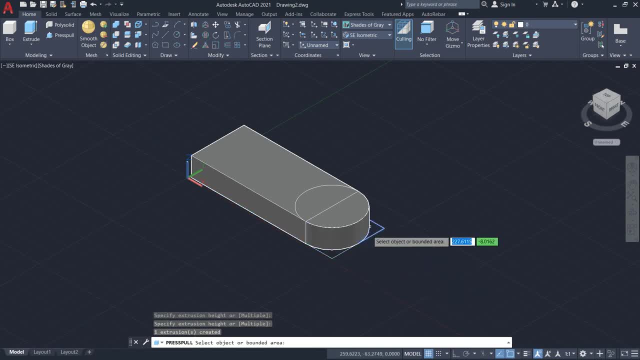 deleted, deleted. so again, I will select this part and go down. okay, you can see this part and go down. okay, you can see this part and go down. okay, you can see, this part is also deleted, deleted. so now this part is also deleted, deleted. so now this part is also deleted, deleted. so now I will draw the inner circle, okay, here. 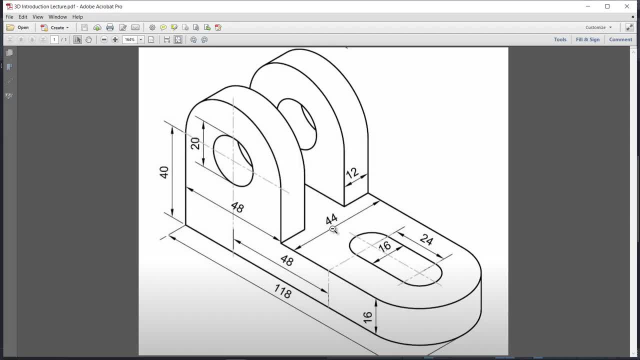 I will draw the inner circle. okay here. I will draw the inner circle. okay here. inner circle dimension is that is 16, so inner circle dimension is that is 16. so inner circle dimension is that is 16. so this circle dies 16 and this circle dies. 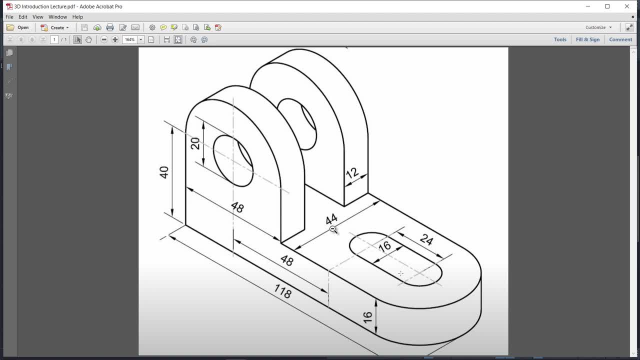 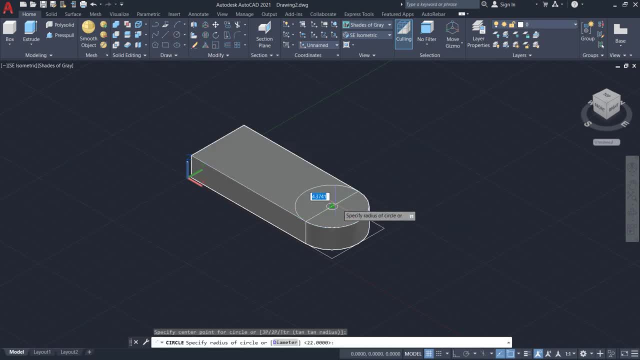 this circle dies 16 and this circle dies. this circle dies 16 and this circle dies 16 and radius will be 8. okay, and now I 16 and radius will be 8. okay, and now I 16 and radius will be 8- okay, and now I will draw the circle, at this point, whose? 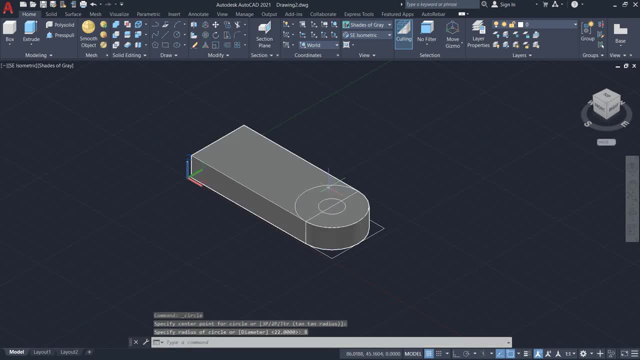 will draw the circle at this point. whose will draw the circle at this point? whose radius is 8? okay, so I want I will copy: radius is 8. okay, so I want I will copy: radius is 8. okay, so I want I will copy this circle. okay, copy and move this. 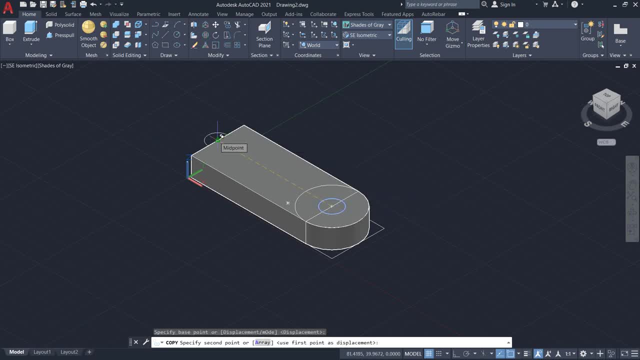 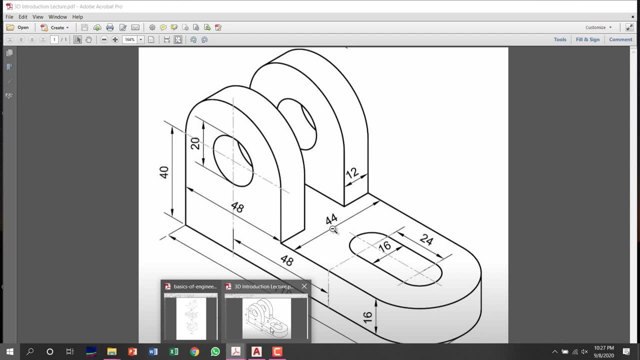 this circle: okay, copy and move this. this circle: okay, copy and move this circle from this position to 24 length. circle from this position to 24 length. circle from this position to 24 length. okay, because the distance between two. okay because the distance between two. okay, because the distance between two circles is 44. 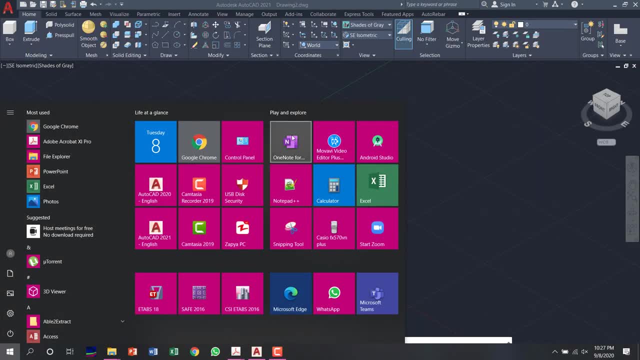 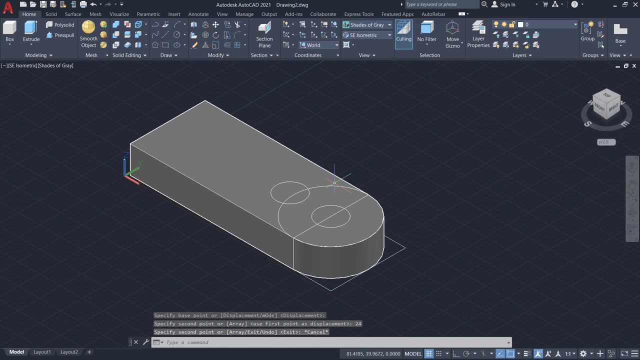 circles is 44. circles is 44- 24. so that's why I have entered 24- okay, 24. so that's why I have entered 24- okay, 24. so that's why I have entered 24- okay. so now I will delete the circle, if you. 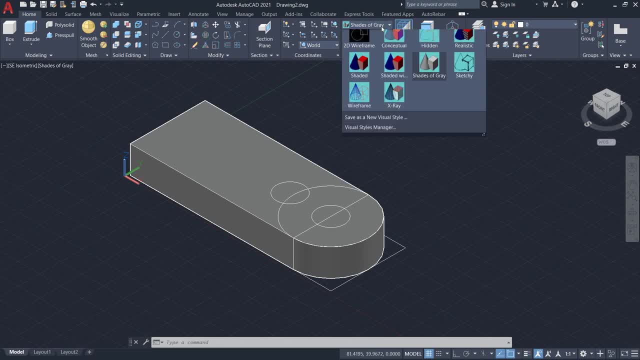 so now I will delete the circle. if you so, now I will delete the circle. if you face any difficulty in selection, you can face any difficulty in selection. you can face any difficulty in selection. you can go back again the 2d wireframe. then you go back again the 2d wireframe, then you. 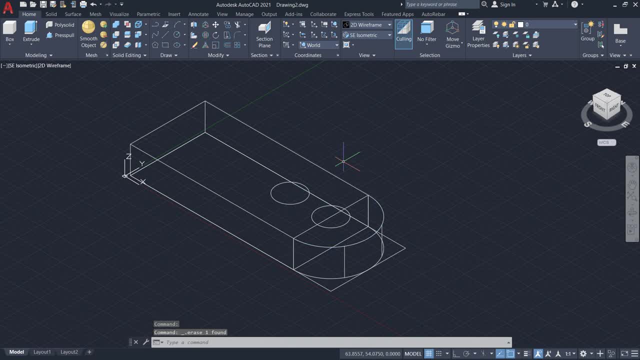 go back again the 2d wireframe, then you will easily select that circle here, I will easily select that circle here. I will easily select that circle here, I will delete. so now I will draw a simple, will delete. so now I will draw a simple, will delete. so now I will draw a simple rectangle. okay, from this point 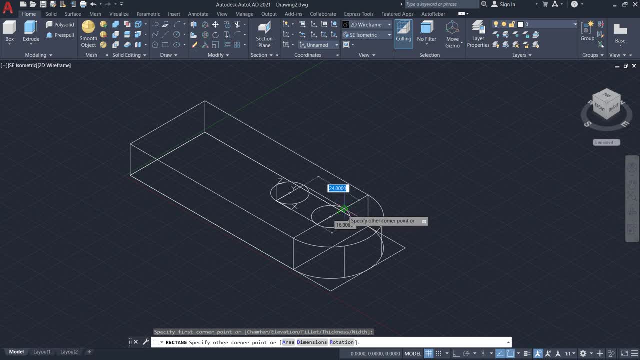 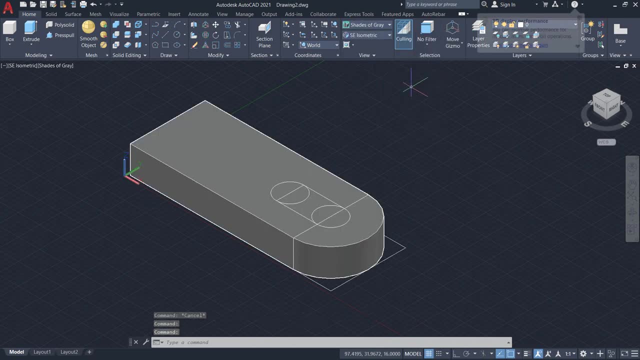 rectangle, okay, from this point. rectangle, okay, from this point to this point. okay, why I have selected the to this point. okay, why I have selected the to this point. okay, why I have selected the rectangle here in the 3d concept. okay, rectangle here in the 3d concept, okay. 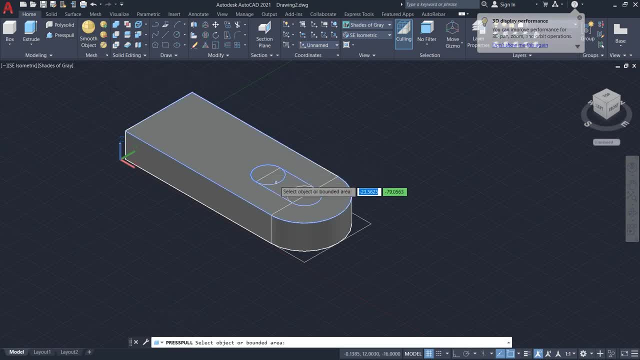 rectangle here in the 3d concept. okay, I will again select, press and pull. I will again select, press and pull. I will again select, press and pull, select that object and go down. similarly, select that object and go down. similarly, select that object and go down. similarly, select that subject, go down in this one. 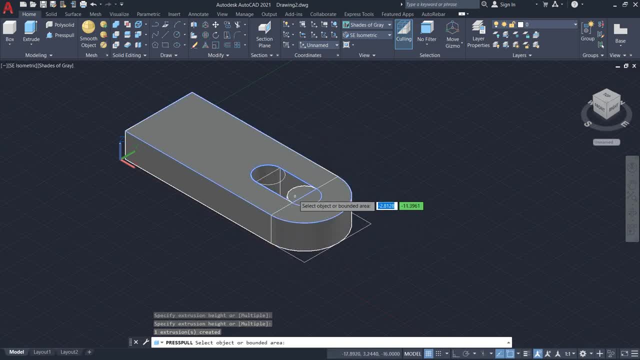 select that subject: go down in this one. select that subject: go down in this one. you can go up. you can go down for. you can go up. you can go down for. you can go up. you can go down for delete and up for delete and up for. 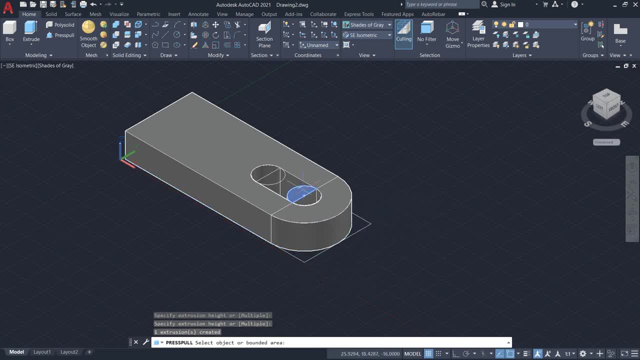 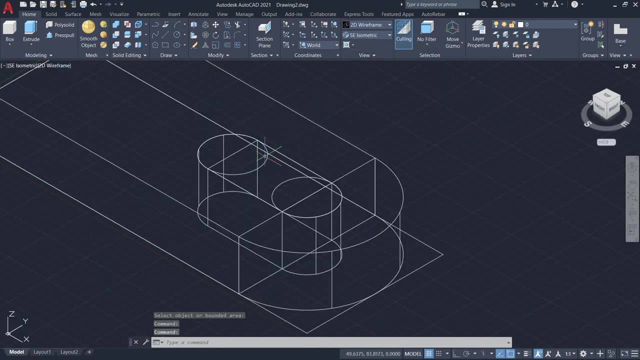 delete and up for projection here. so now I do not need these inner projection here. so now I do not need these inner projection here. so now I do not need these inner circles. so I will go select, select circles. so I will go select select circles. so I will go select, select, select, delete. okay, again, go back in the 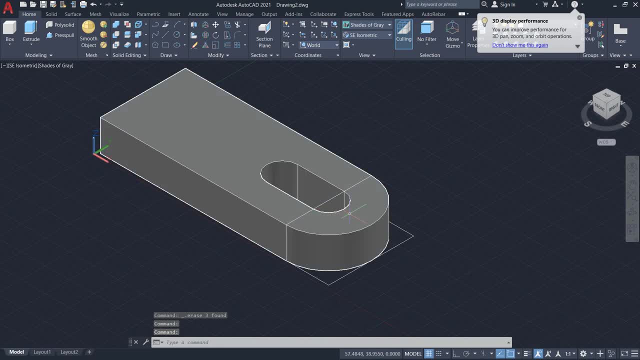 select delete. okay again, go back in the select delete. okay, again, go back in the shaded view. okay, now you can see I have shaded view. okay, now you can see I have shaded view. okay, now you can see I have drawn the inner elliptical part. okay, I. 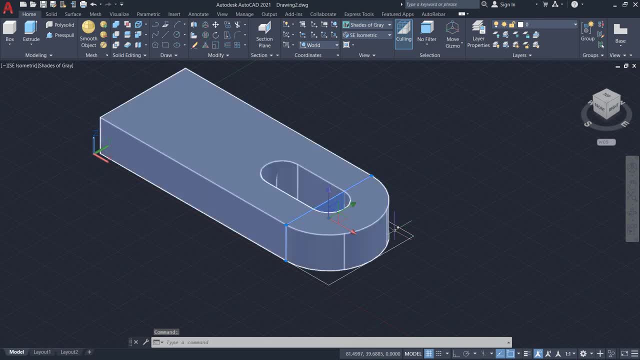 drawn the inner elliptical part. okay, I drawn the inner elliptical part. okay, I will select this face which I have copied. will select this face which I have copied. will select this face which I have copied. and we also do not need this bottom and we also do not need this bottom. 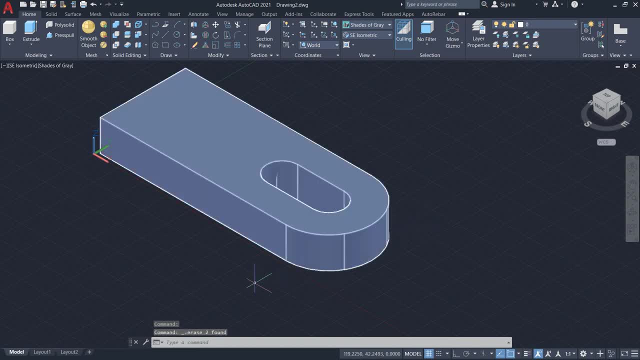 and we also do not need this bottom reference point. so I have deleted all reference point. so I have deleted all reference point. so I have deleted all these. so now I will draw the upper part, these. so now I will draw the upper part, these. so now I will draw the upper part. okay, the upper part, whose dimension is: 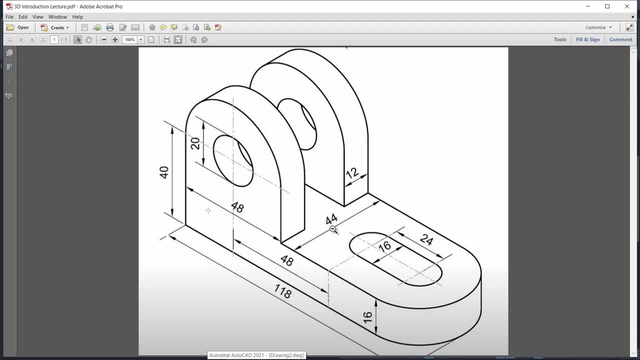 okay, the upper part whose dimension is okay. the upper part whose dimension is from this point to upward. so width is 48 from this point to upward. so width is 48 from this point to upward. so width is 48 and thickness is 12 and the height from. 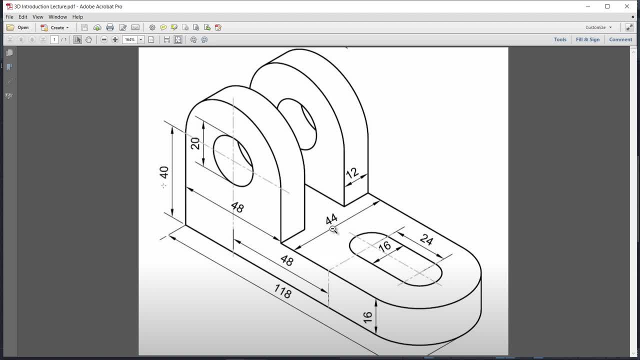 and thickness is 12 and the height from and thickness is 12 and the height from this point to this point. so if we 40 this point to this point, so if we 40 this point to this point, so if we 40 subtract this 16, then the distance from: 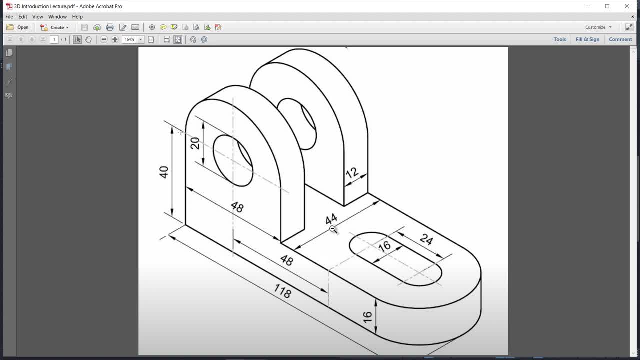 subtract this 16, then the distance from subtract this 16, then the distance from this point to this point will be 24, and this point to this point will be 24, and this point to this point will be 24. and this is the curve. so the radius, the dia. 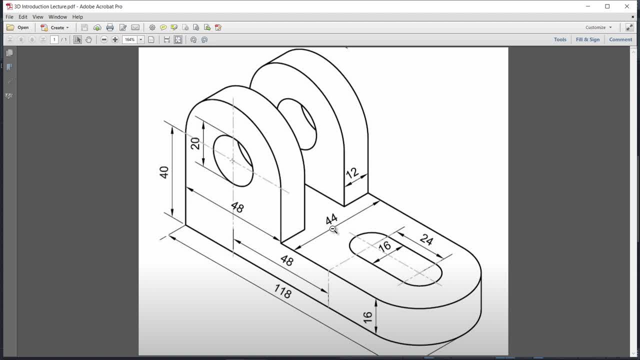 this is the curve, so the radius, the dia. this is the curve, so the radius, the dia is also 48, so radius will be 24, so 24. 24 is also 48, so radius will be 24, so 24. 24 is also 48, so radius will be 24, so 24, 24. this from this point to this point, 24. 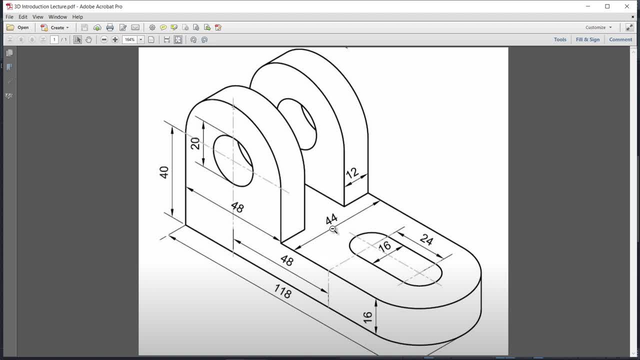 this: from this point to this point 24. this, from this point to this point 24. from this point to this point 24, 48. so from this point to this point 24, 48. so from this point to this point 24, 48. so that is the 48 by 48 panel with. 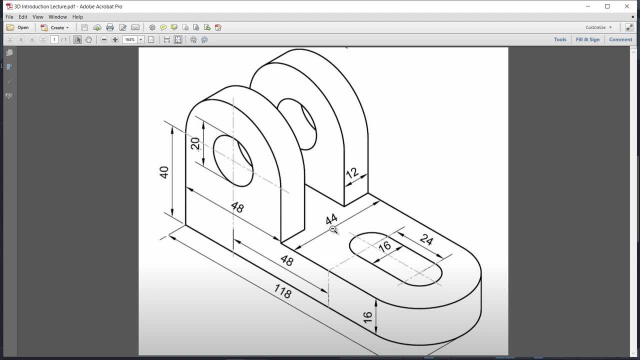 that is the 48 by 48 panel with. that is the 48 by 48 panel with thickness 12, and here the again with thickness 12, and here the again with thickness 12, and here the again with small diameter circle of 20. okay, now I. 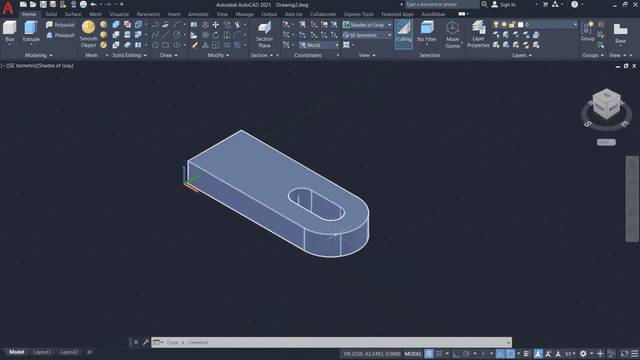 small diameter circle of 20. okay, now I. small diameter circle of 20. okay, now I will show this. okay, I, now I will select, will show this. okay, I now I will select, will show this. okay, I now I will select. and the coordinate system in which I 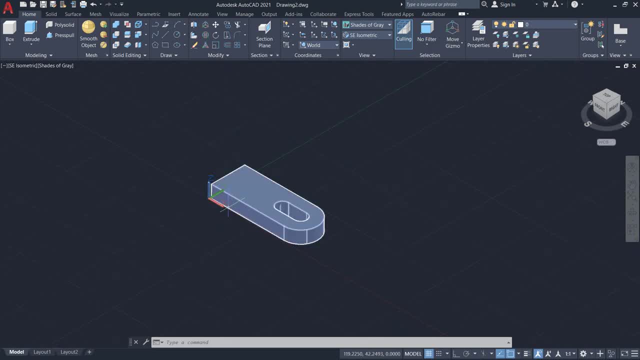 and the coordinate system in which I and the coordinate system in which I want to work, so if I want to work in, want to work, so if I want to work in, want to work, so if I want to work in this phase, in the left phase, so you can. 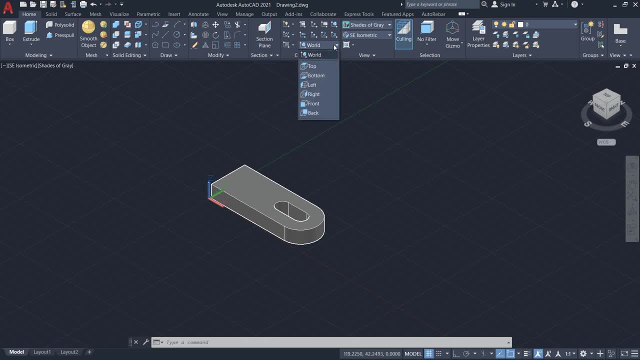 this phase in the left phase, so you can this phase in the left phase, so you can select any phase. okay here. if you want select any phase, okay here. if you want select any phase, okay here. if you want to work the entire phase bottom left, to work the entire phase bottom left. 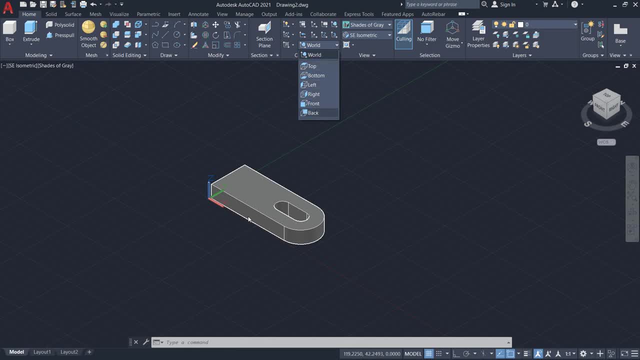 to work the entire phase bottom left, right back. so this is my front face. so I right back. so this is my front face. so I right back. so this is my front face. so I will select this front now if I draw any. will select this front now if I draw any. 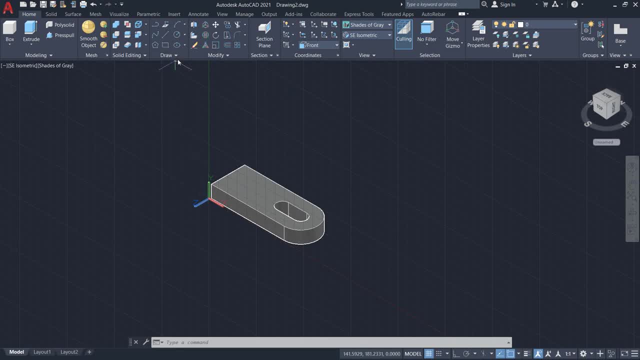 will select this front. now, if I draw any dimension, that will work in the front dimension. that will work in the front dimension. that will work in the front phase. so here I will draw again phase. so here I will draw again phase. so here I will draw again rectangle. select any point. okay, I have. 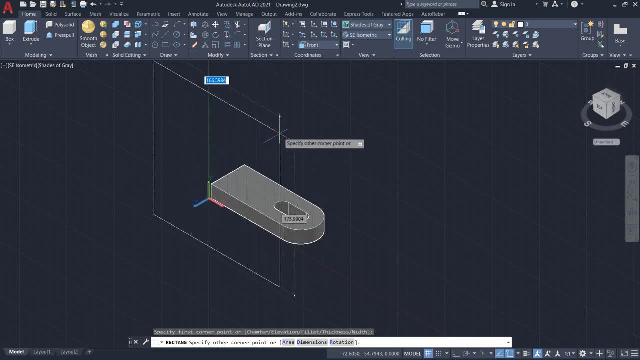 rectangle select any point. okay, I have rectangle: select any point. okay, I have selected any point. now you can see I am selected any point. now you can see I am selected any point. now you can see I am drawing the dimensions in the front face. drawing the dimensions in the front face. 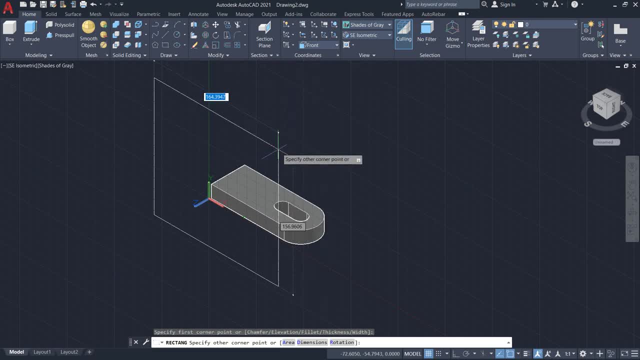 drawing the dimensions in the front face. due to the coordinate system in the. due to the coordinate system in the. due to the coordinate system in the previous version of our two cats- this previous version of our two cats, this previous version of our two cats- this option of coordinate system is present. 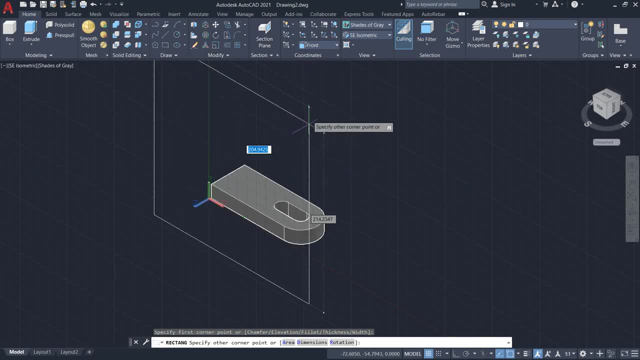 option of coordinate system is present. option of coordinate system is present in the view tab. okay, in the advanced in the view tab. okay in the advanced in the view tab. okay in the advanced autocad version. that is present in the autocad version. that is present in the. 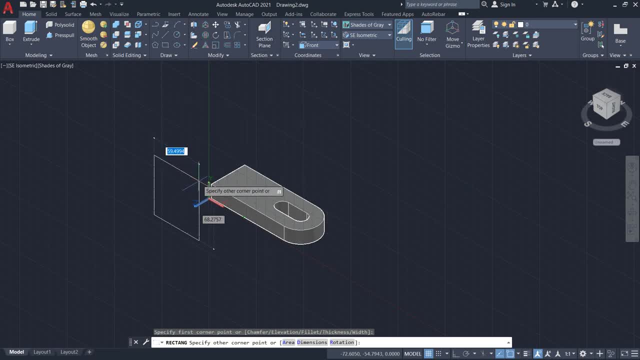 autocad version that is present in the main home button. okay, so now I will main home button. okay, so now I will main home button. okay, so now I will enter the dimensions width is 48 and enter the dimensions width is 48 and enter the dimensions width is 48 and height is also 48. okay, now I will press. 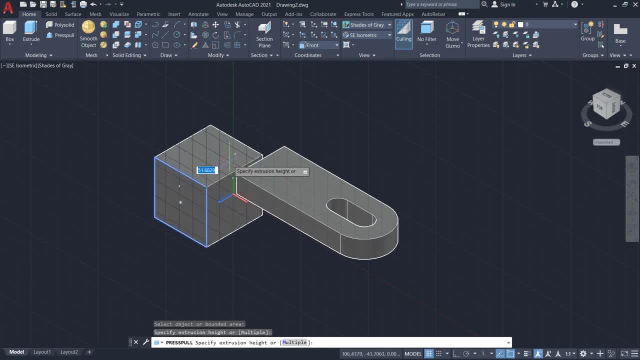 height is also 48. okay, now I will press. height is also 48. okay, now I will press and pull. okay, press and pull how much. and pull- okay, press and pull how much. and pull- okay, press and pull how much- 12. and now I will draw the circle. 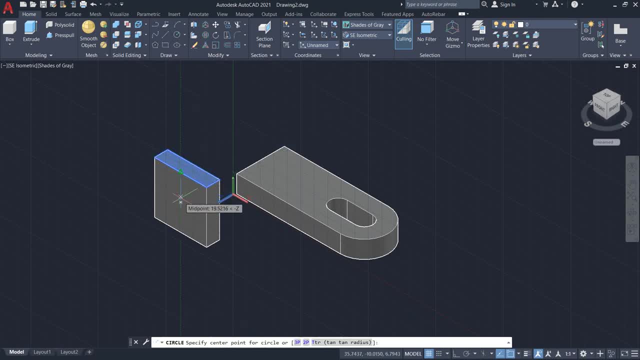 12 and now I will draw the circle. 12 and now I will draw the circle. okay for the drawing of circle. I need the okay for the drawing of circle. I need the okay for the drawing of circle. I need the center. I will just snap that set. 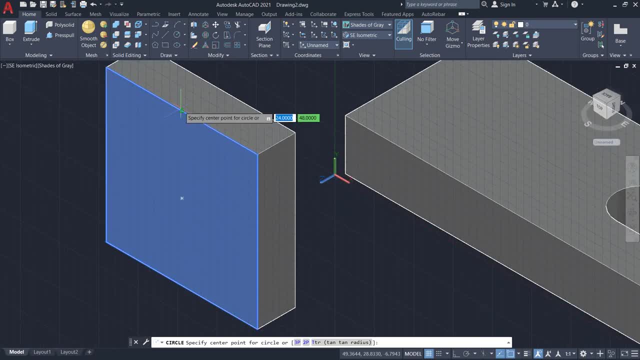 center. I will just snap that set center. I will just snap that set Center. okay, now I will draw this circle Center. okay, now I will draw this circle Center. okay, now I will draw this circle. okay, delete, I will create the upper. okay, delete, I will create the upper. 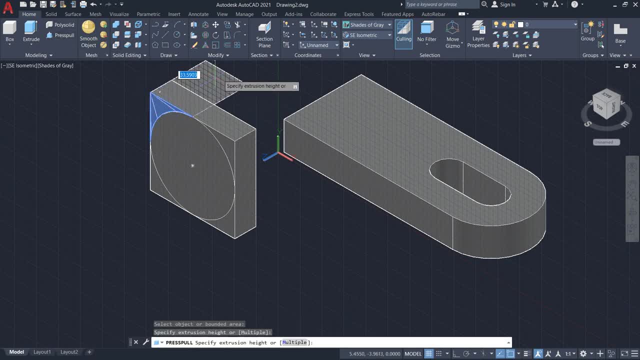 okay, delete. I will create the upper parts by using press and pull. okay, now I parts by using press and pull. okay, now I parts by using press and pull. okay, now I will draw the inner circle. whose will draw the inner circle? whose will draw the inner circle whose diameter is 20? okay, first of all, I will 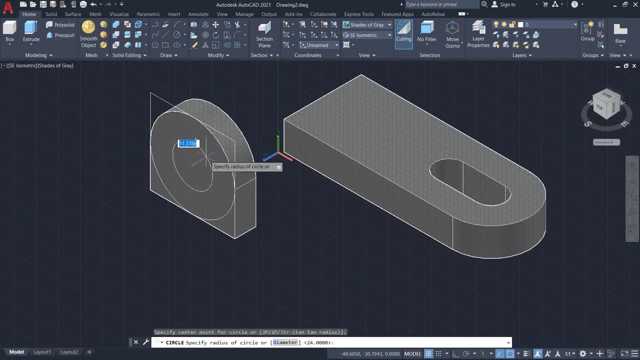 diameter is 20. okay, first of all, I will. diameter is 20: okay, first of all, I will snap the center now I will enter. snap the center now I will enter. snap the center now I will enter. the radius radius will be 10. now I will. 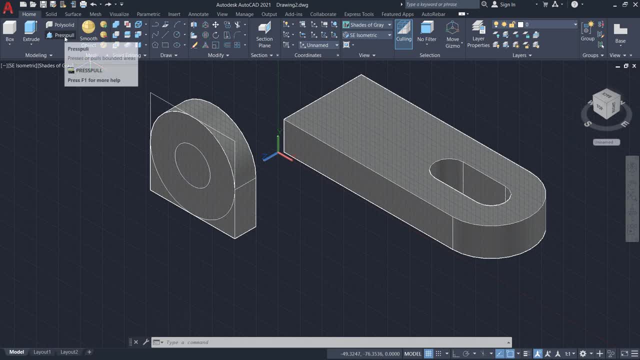 the radius radius will be 10. now I will. the radius radius will be 10. now I will delete the inner circle. okay, select, delete the inner circle. okay, select, delete the inner circle. okay, select, press and pull and remember for press. press and pull and remember for press. 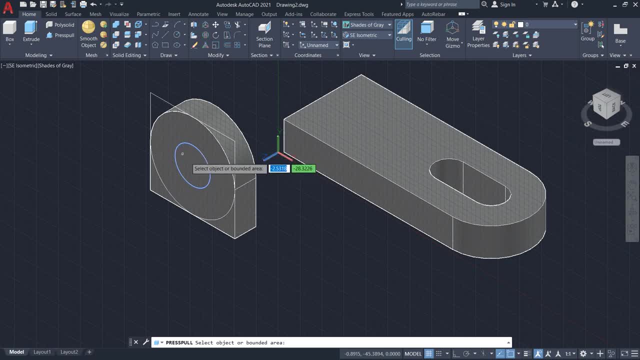 press and pull and remember, for press and pull, you have to select the inner and pull. you have to select the inner and pull. you have to select the inner surface. note the edges. okay, I will surface. note the edges. okay, I will surface. note the edges. okay, I will select this surface and go inward. okay, I. 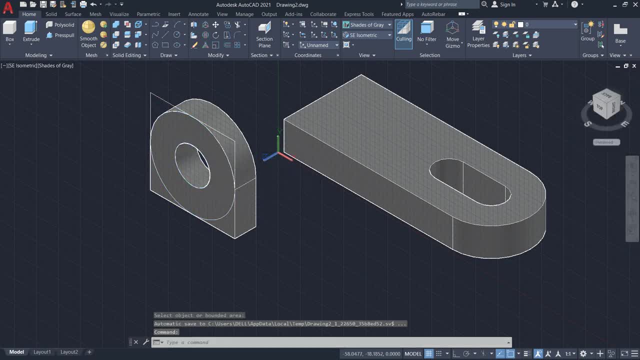 select this surface and go inward. okay, I select this surface and go inward. okay, I have deleted, so now I will delete this. have deleted, so now I will delete this. have deleted, so now I will delete this portion also and this circle outline portion also, and this circle outline. 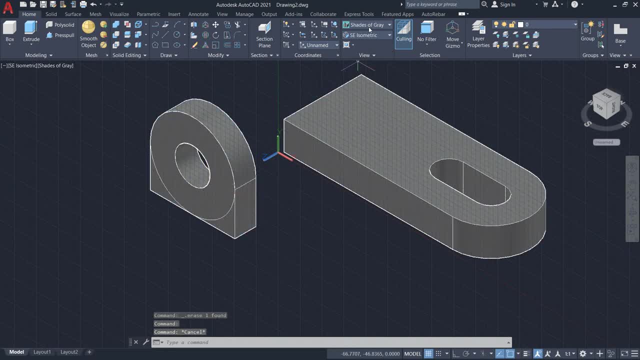 portion also and this circle outline. okay, here I am facing the issue in. okay, here I am facing the issue in. okay, here I am facing the issue in selection. so I will go in the 2d frame I- selection. so I will go in the 2d frame I. 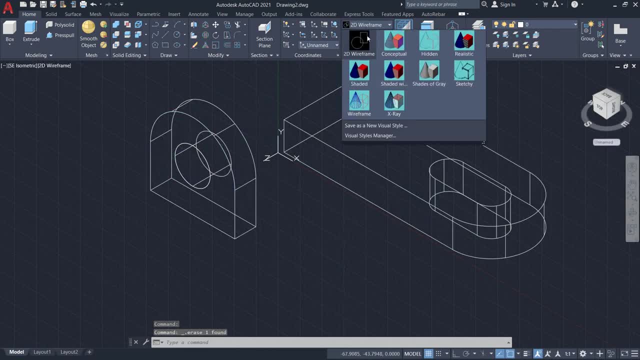 selection. so I will go in the 2d frame. I will select, just select, delete again. go will select, just select, delete again. go will select, just select, delete again. go to shaded view. now I have to copy the to shaded view. now I have to copy the.